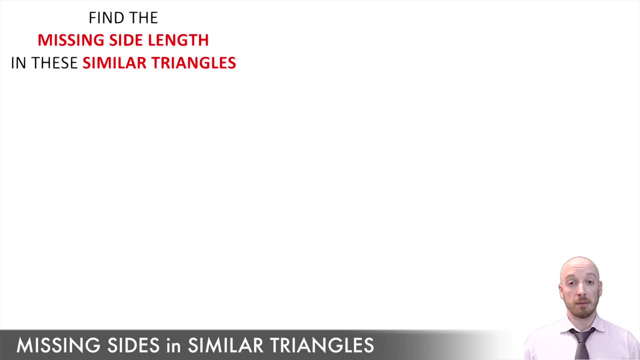 question like this on an exam. First up, they love to show similar triangles that are vertically opposite to each other. Now, the first thing we have to do here, as in any question with similar triangles, is identify the angles that are the same in these two triangles. So I'm going to go ahead and label my 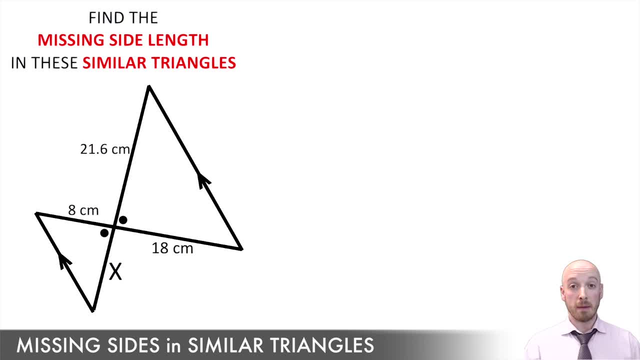 vertically opposite angles as matching angles And then- remember, these are alternate interior angles that I'm going to label next. So in opposite corners of the transversals, where they meet the parallel lines, I have my other pairs of matching angles And watch as I redraw these triangles beside each other. the 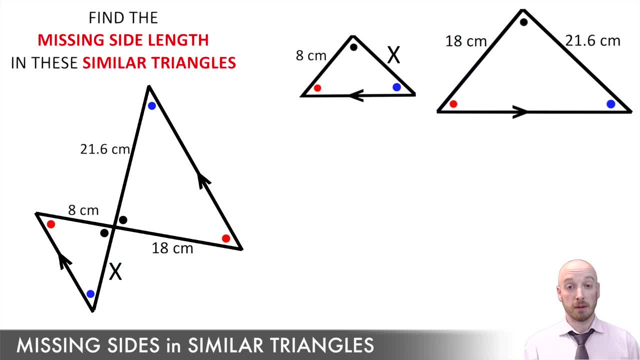 orientations change a little bit. It's important that you put the matching angles in the same place when you sketch these triangles yourself. Now, with the triangles redrawn properly, we can identify easily where the corresponding sides are. So I'm going to go ahead and do that. 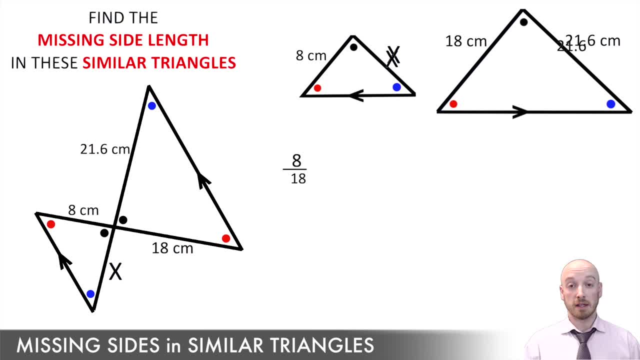 So I'm going to set up my fractions with corresponding sides and solve for the unknown. All I need to do here is multiply the diagonals and then divide by what's in front of X to find out that that missing side length we were looking for is 9.6 centimeters. Now, the math here was pretty. 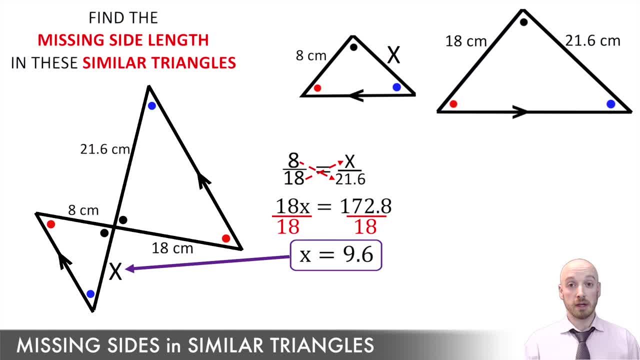 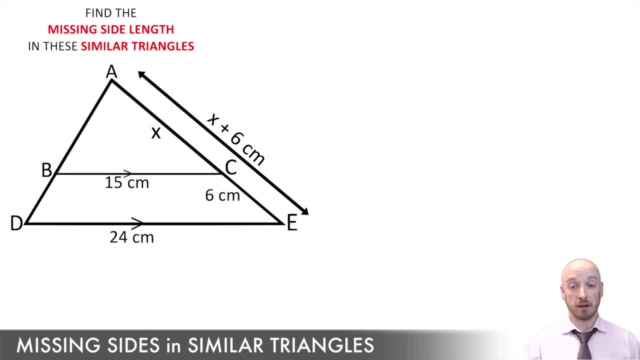 easy, but setting up this question is what's tricky. You've got to make sure you get the orientation right and find those pairs of matching angles. Now, in this next question, the setup is a little different And the math is going to be quite a bit tougher. So pay close attention here. 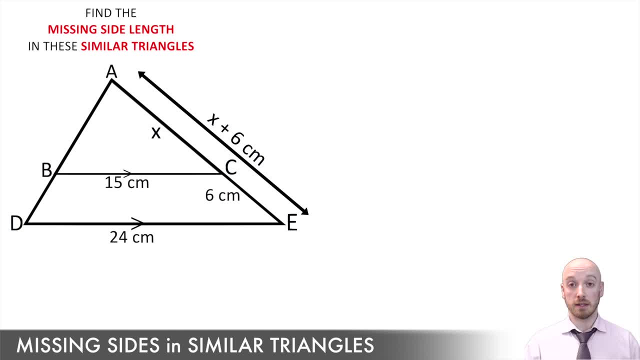 What we've got are two triangles, one drawn right inside the other, with the top angles lined up and the bases being identified as parallel lines. Now, what I'm going to do here is redraw these two triangles separately, like we always do, with the matching angles identified, so the corresponding sides become obvious. 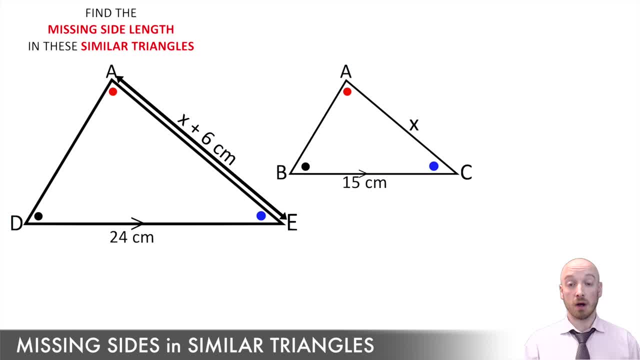 Now, once this is done, we can get started by setting up the obvious proportion, And this one is that 15 and 24 are corresponding sides. So I'm going to go ahead and do that. So I'll use that as my first fraction: 15 over 24.. So my second fraction has to get. 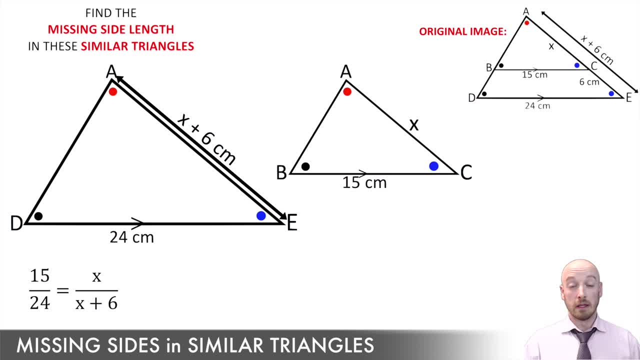 set up as X over X plus 6.. Now it looks like we might be stuck here. but don't panic, Let's multiply it out and see what we can do. And when I multiply the diagonals here, I get 24 times X, and then I get 15 times X plus 6.. Now be careful. 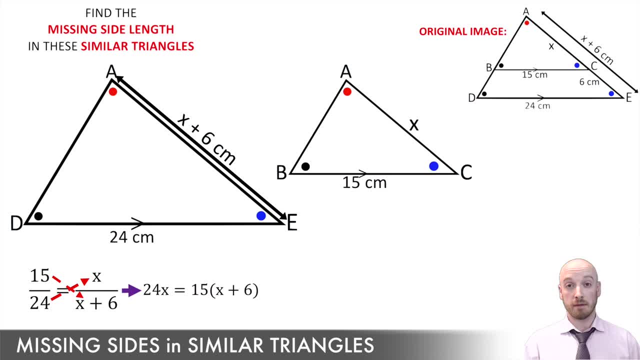 here and remember: when I've got a number multiplied by two terms, I've got to multiply the number out front by the two terms separately that I've got. So here I'll do 15 times X and then 15 times 6.. Now, once I do all this, what I end up? 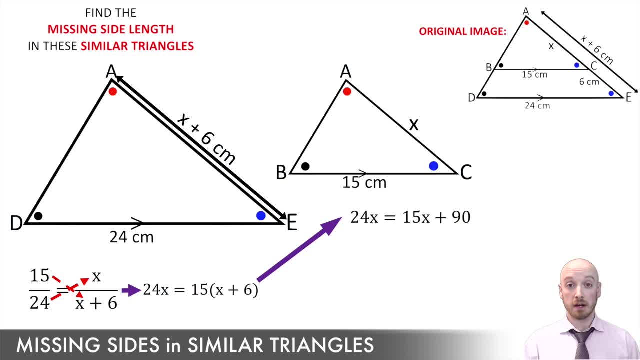 with on the left side is 24X, and on the right side I've got 15X plus 90. Now this is actually not so bad. All I'm going to do here is gather my X terms on one side of equals by subtracting 15X from both sides, And look how easy this is. All I'm left with is 9X. 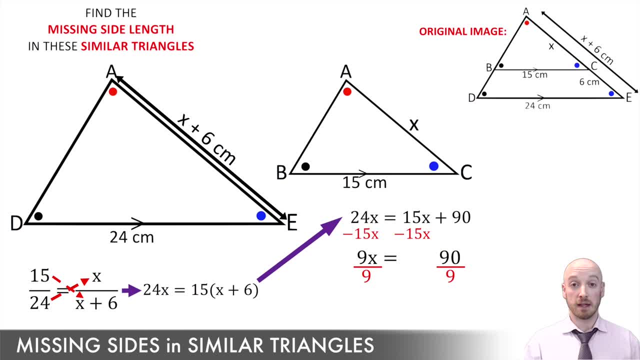 equals 90. So I'm going to go ahead and divide by that 9 in front of X to get the X by itself. Of course, I've got to divide by 9 on the other side as well, And what I'm left? 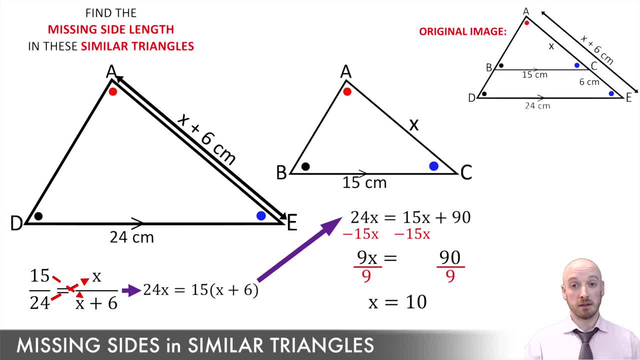 with is X equals 10.. So the missing measurement that they were looking for in this question, side AC of that smaller triangle- is just a measurement of 10 centimeters. So when you're finding missing side lengths in similar triangles, remember find your corresponding sides, set up your. 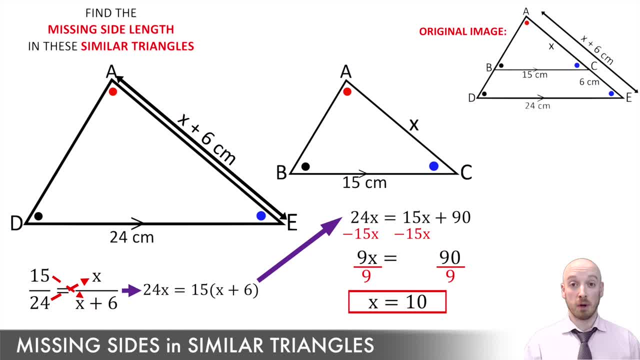 fractions and just be careful with your algebra. We're going to cross, multiply to find that unknown value. Now let's watch a couple more examples on how they might ask these types of questions. 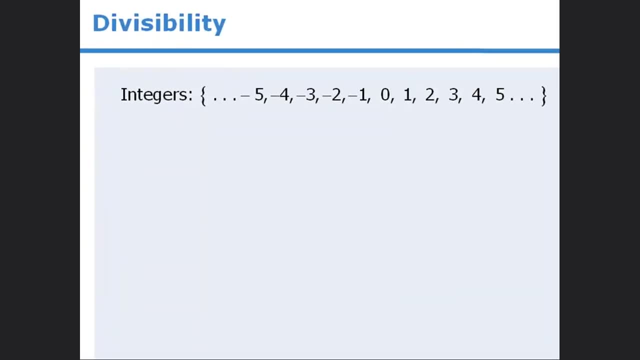 Welcome to the first lesson of the Integer Properties module. Now, in a nutshell, the topic of Integer Properties is largely related to how the composition of an integer affects its characteristics and the way it behaves. One of the central themes of Integer Properties is divisibility If x and y are integers. 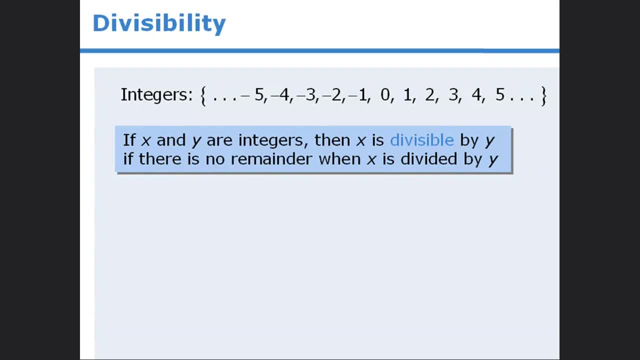 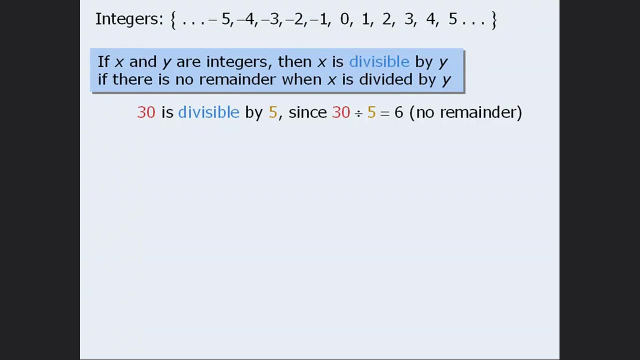 then we say that x is divisible by y if there is no remainder. when x is divided by y, A generative subset is ABench. Similarly, 12 is divisible by 3, since 12 divided by 3 is equal to 4, with no remainder. 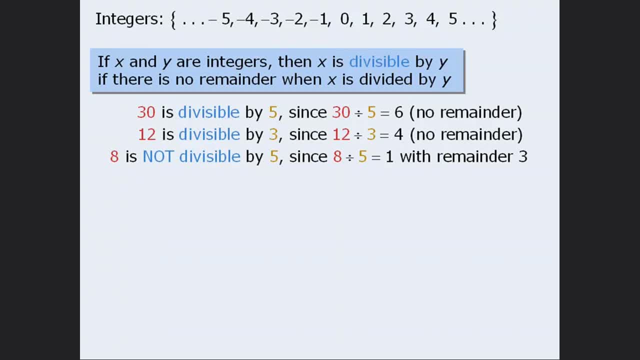 Conversely, 8 is not divisible by 5, since 8 divided by 5 is equal to 1, with remainder 3.. Another way to define divisibility is to say that if x and y are integers, then we say that x is divisible by 5..